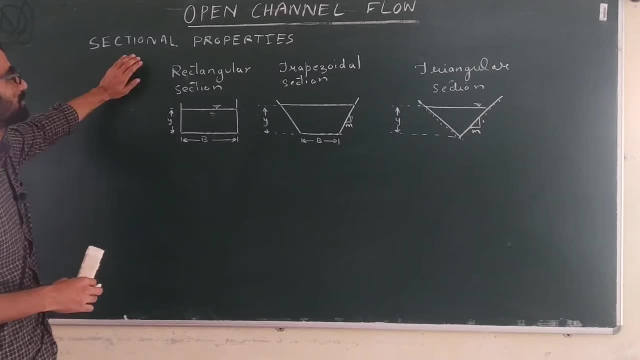 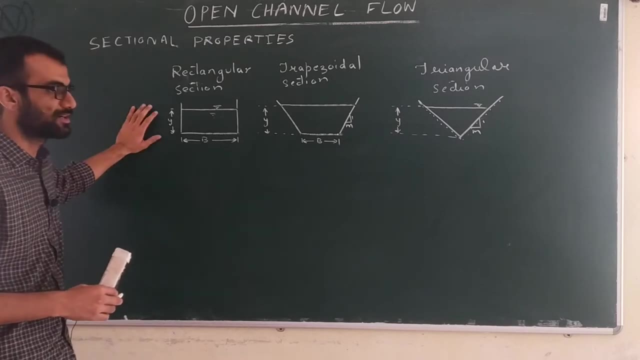 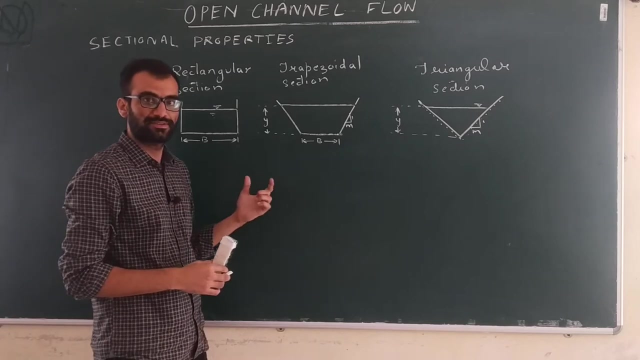 Hello everyone. So today we are going to talk about the sectional properties, or the properties of open channel flow sections. These properties are required to solve the open channel flow problems, So we will discuss the properties simultaneously and we will find out the expressions for those properties for these three commonly encountered sections. So first is a rectangular. 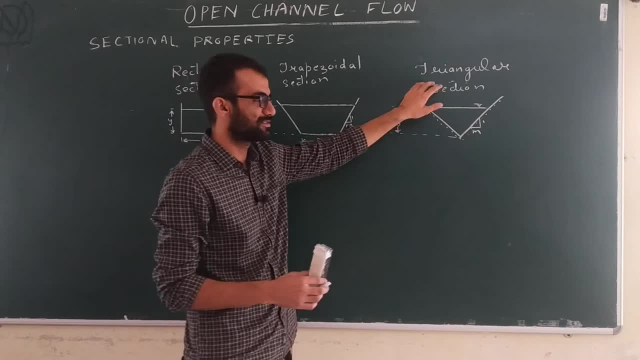 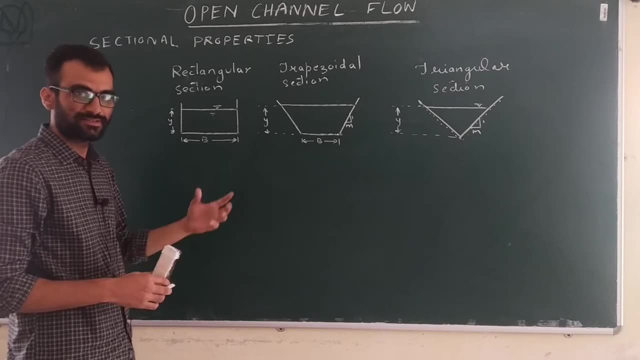 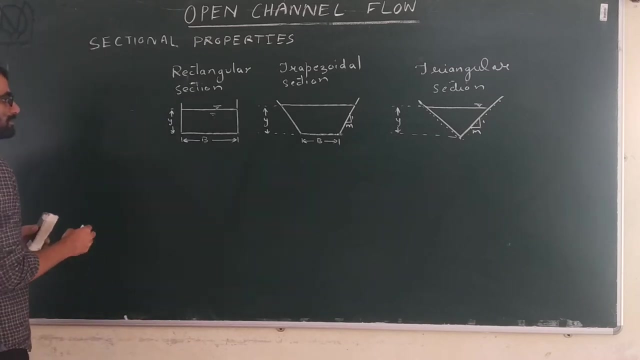 cross section, second is a trapezoidal cross section and third is a triangular section. So these basic sections, if we try to do the expressions. the rest of the sections you can easily calculate from the idea of this, previous sections. So first we will see what. 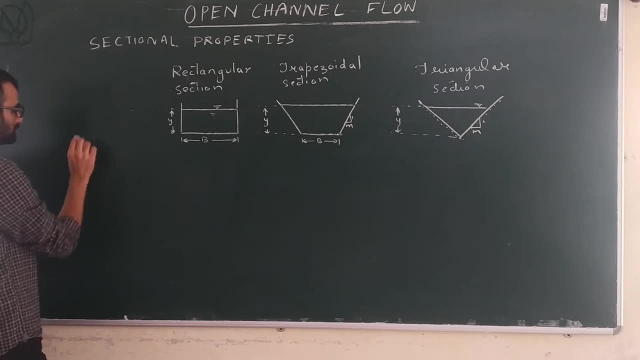 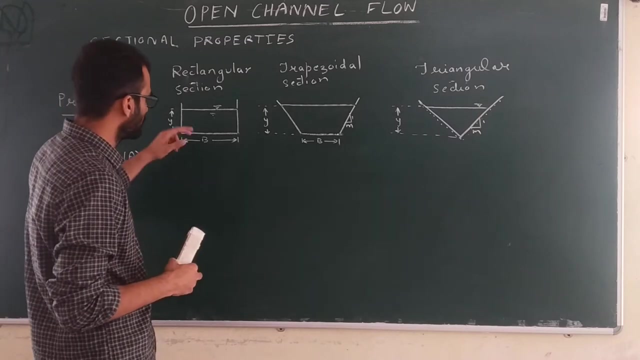 is the first property or sectional property that we will see. that is the flow area. So flow area it is denoted by capital A. Generally, flow area is denoted by capital A. So what do you mean by flow area? Flow area is the cross sectional area of the flow, normal to. 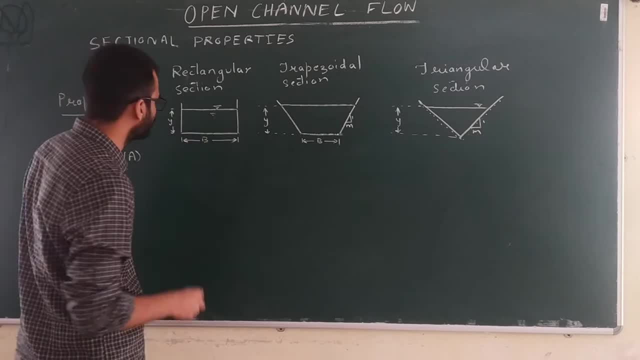 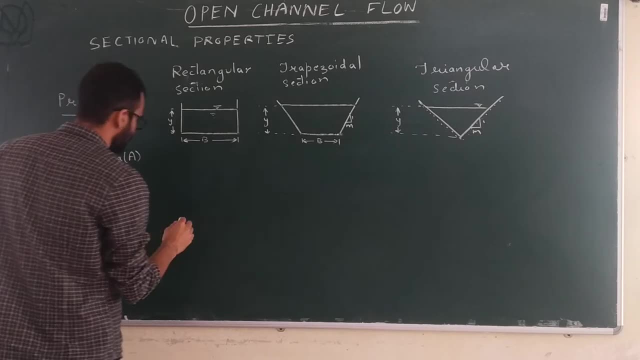 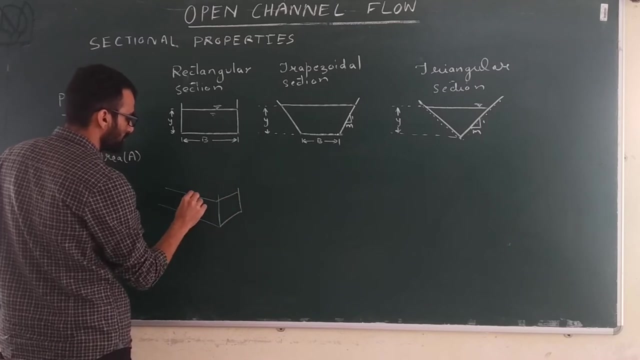 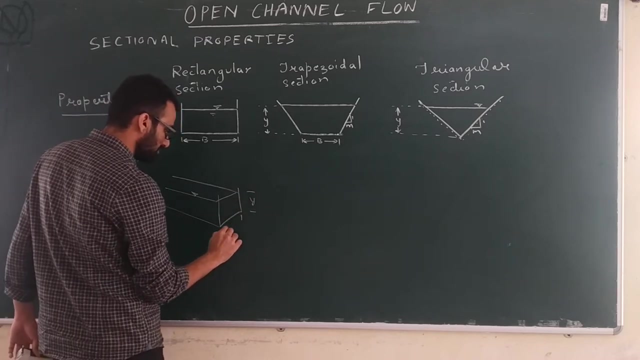 the flow depth normal to the direction of the flow. So if flow is taking place like this, you know, So flow is taking place. if you want to draw this rectangular cross section, if you have flow is taking place like this, this is your flow depth. flow is taking place. So this is the depth of flow and this is the width. 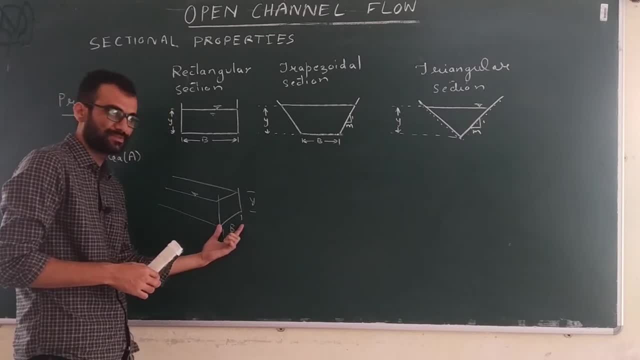 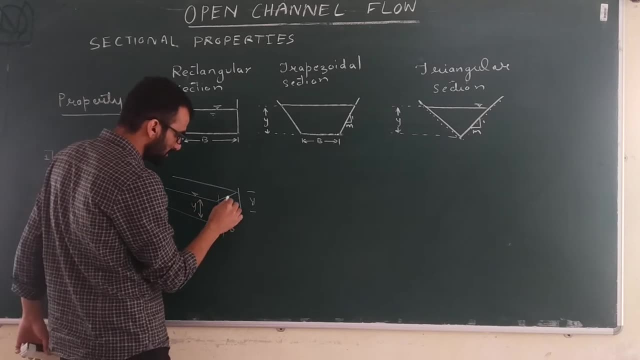 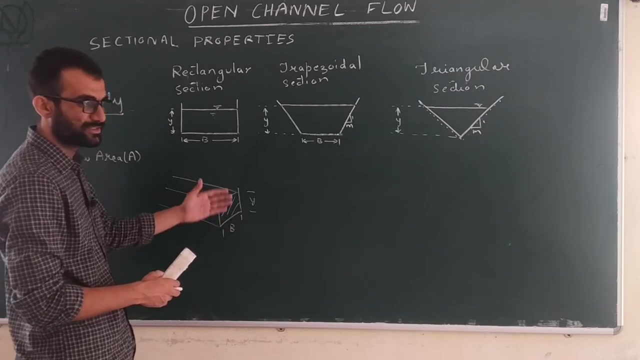 of section. This is the width, base width- and flow is taking place. this is the depth. So what will be the cross sectional area of the flow? It will be this area of the flow. So if you cut a cross section measure the area through which the flow is taking place, that area is called as the flow area. all. 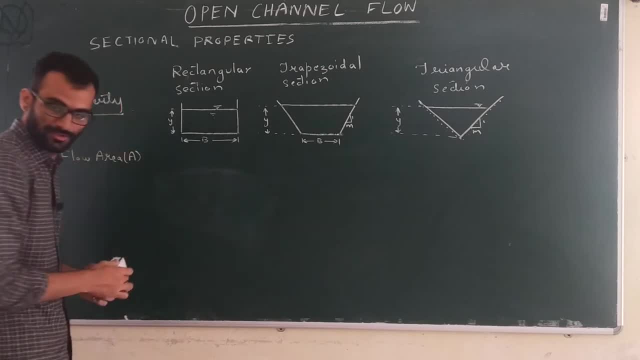 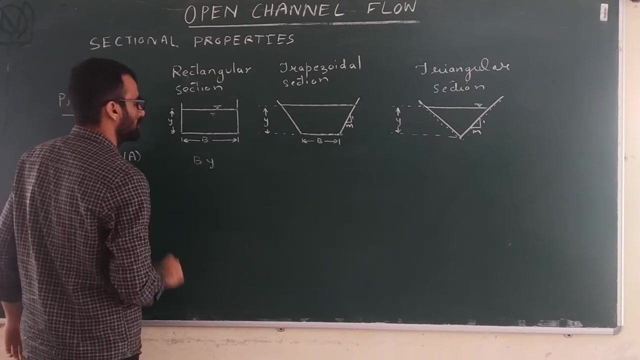 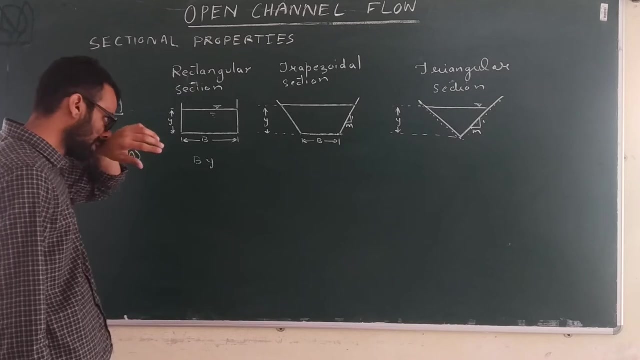 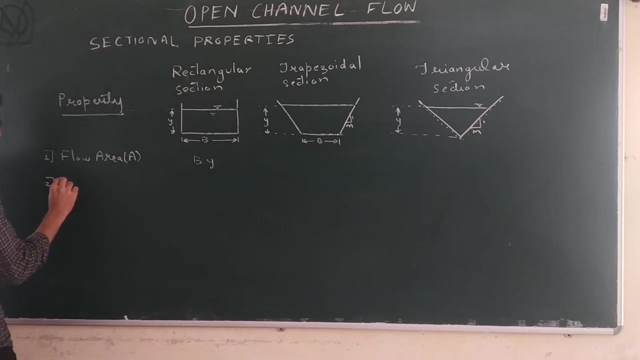 right, so for rectangular cross sections, what will be that flow area for rectangular cross sections? it will be b into y, okay, base width multiplied by flow depth, area of rectangle. that's it. that will be your flow area, okay, now, second property is the wetted perimeter. it is denoted by p, capital, p, okay, so wetted perimeter is basically the. 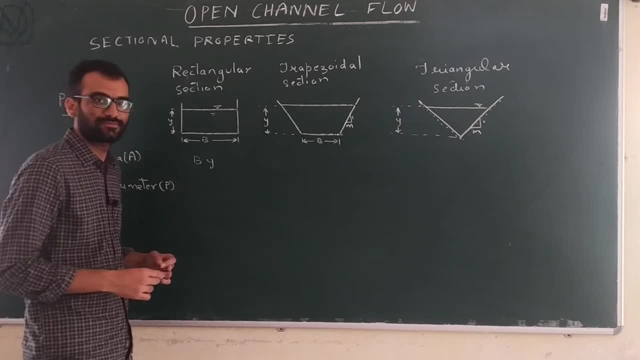 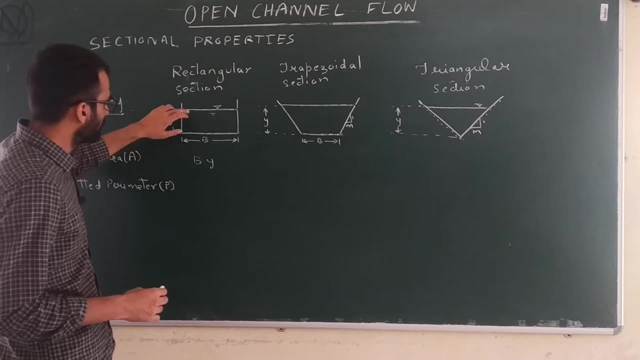 length of the surface that is wetted in the cross-section or flow area. So what is the length of the cross-section which is wetted by the flow? Okay, So the flow is now wetting this surface. Okay, This is the cross-section and this is the 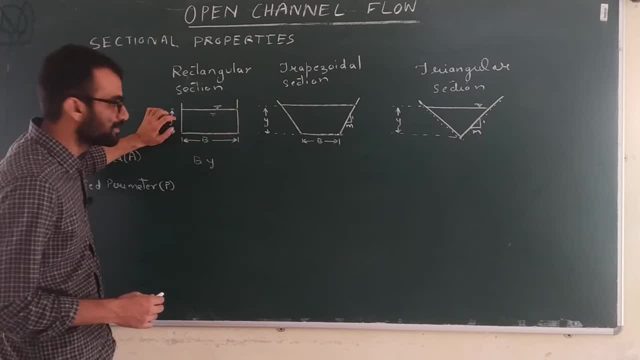 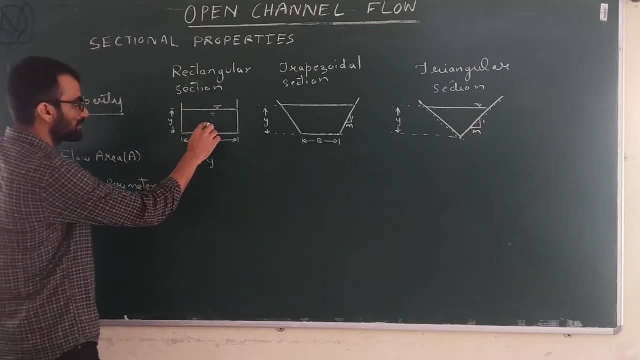 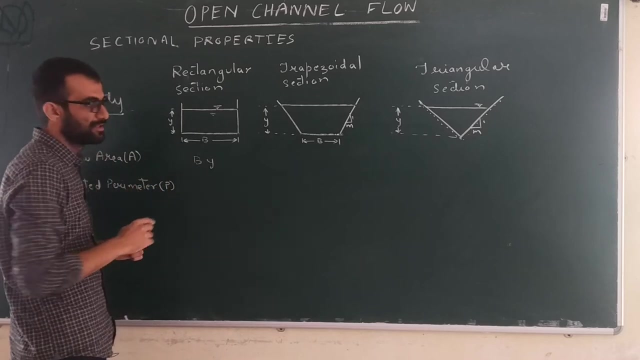 surface for which the fluid is in contact. So how much length of the surface that is in contact with the fluid? that is nothing but the wetted perimeter. Okay, So for rectangular cross-section, what will be that Length? it will be this width plus this height, plus this height, This length. 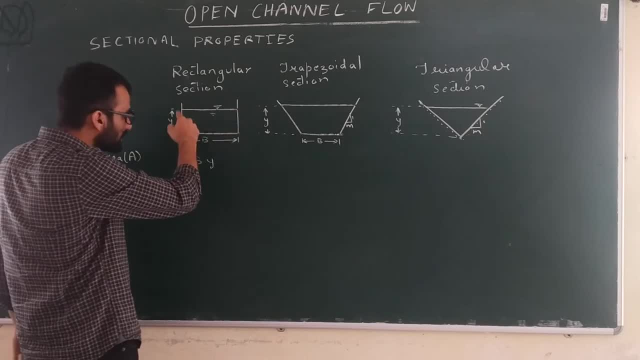 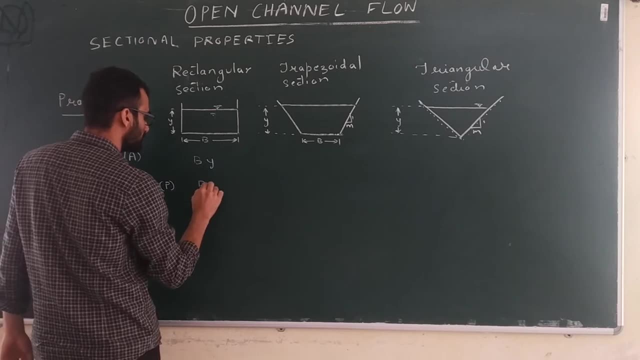 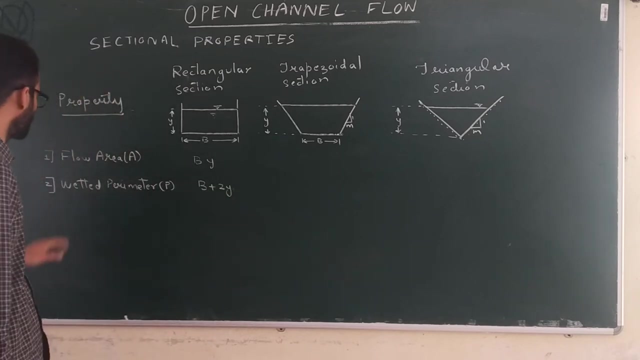 total length is in contact with the fluid, So fluid is wetting this much length of the cross-section, So that is why that is called as the wetted perimeter Now. so here it will be B plus this, Y plus this Y, So B plus twice Y. Okay, So this is your wetted perimeter. 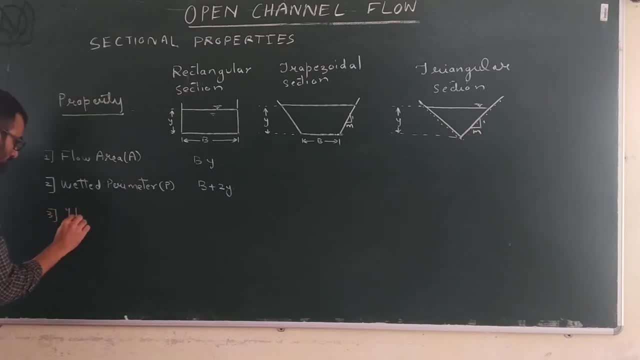 Third is hydraulic radius. It is denoted by capital R. Hydraulic radius is given by A, by P, So hydraulic radius is defined as the ratio of flow area to the wetted perimeter. Okay, That is how you define the hydraulic radius. 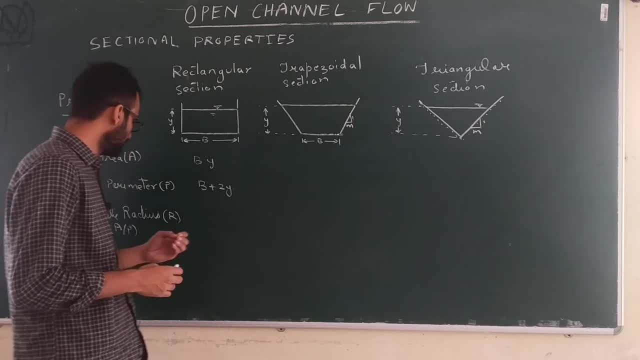 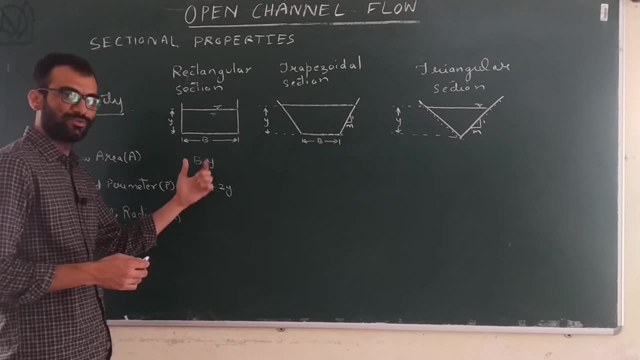 Basically, hydraulic radius becomes, the becomes a, it becomes a characteristic length of a particular flow, open channel flow- when we try to connect it to the wetted perimeter. So this is the wetted perimeter. So if you want to calculate some parameters, Okay, Like the Reynolds number. 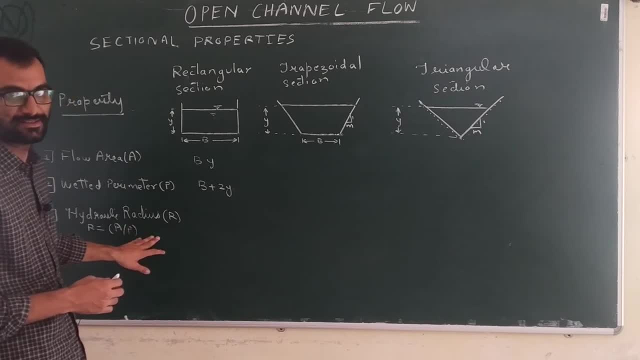 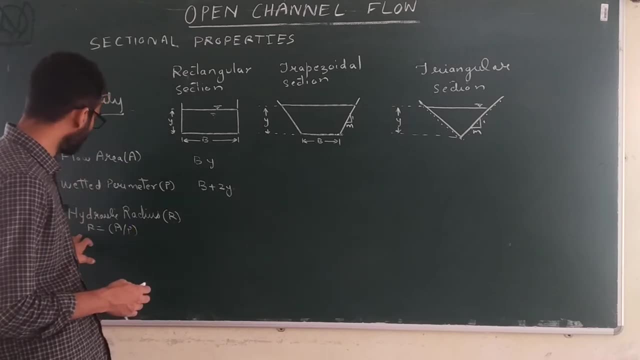 suppose, if you want to calculate, So this becomes the characteristic length. Okay, Like, characteristic length for pipe flow will be the diameter of the pipe. Okay, In the same way, characteristic length can be used, can be taken as hydraulic radius, if we are considering 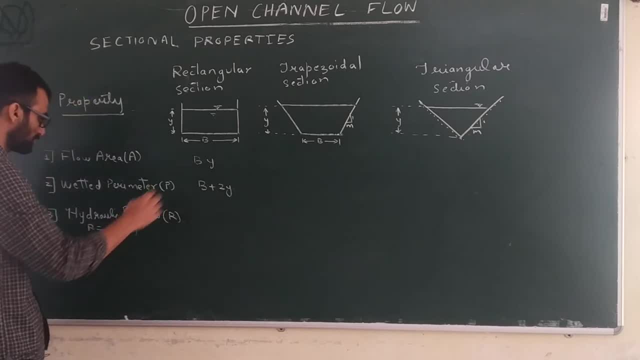 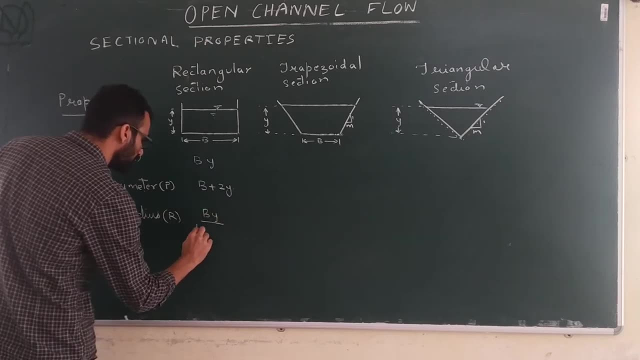 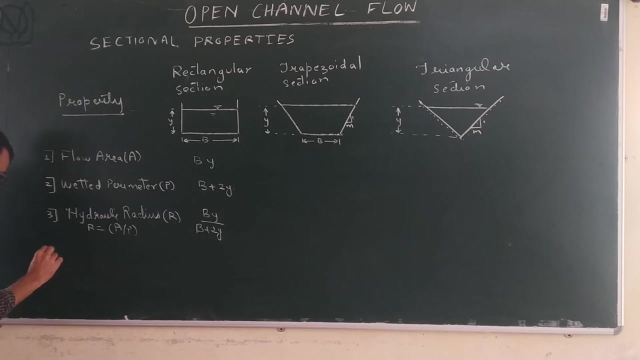 the open channel flow. Alright. So how do so? it will be R equal to A, Y, P. So for rectangular cross-section, it will be B Y upon B plus twice Y. Okay, Because this is the area, this is the perimeter. Then, lastly, you have hydraulic mean. 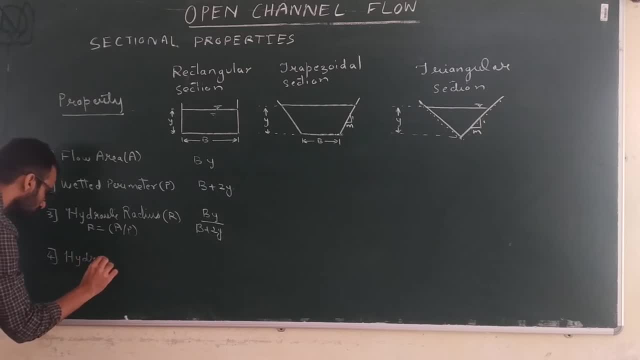 depth or hydraulic depth, simply So, hydraulic depth is denoted as capital D generally, and D is given by A, by T. Okay, So what is this? A by capital T? Capital A is the flow area and T is the top width of the flow. So what is the top width of the flow? So what is the top width of the flow? 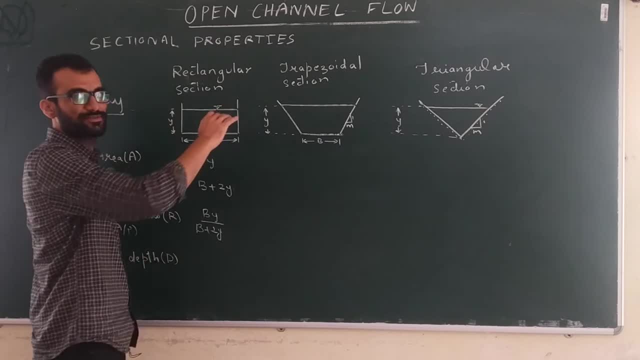 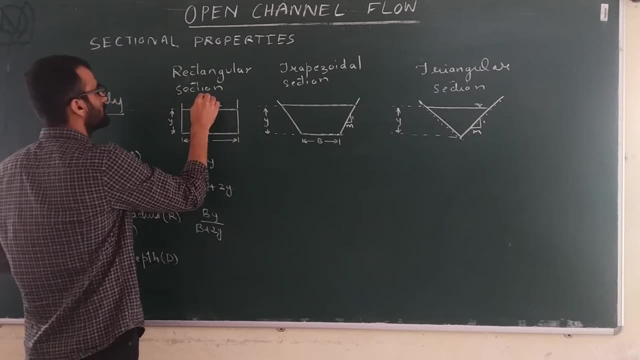 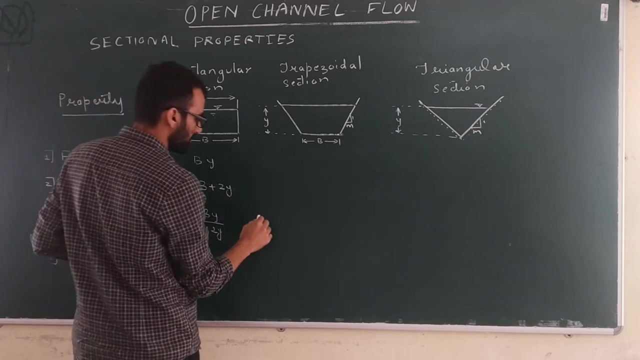 Whenever a flow is taking place, free surface flow is taking place at the free surface, the width, whatever you get the width, that is the top width. So here it is this T. So, anyways, whenever a flow is taking place, let us say: this is a natural cross-section. Okay, A natural. 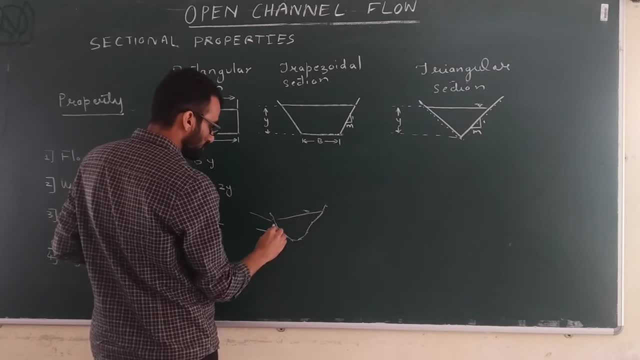 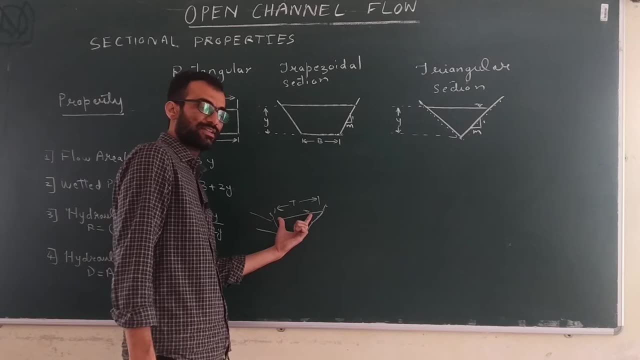 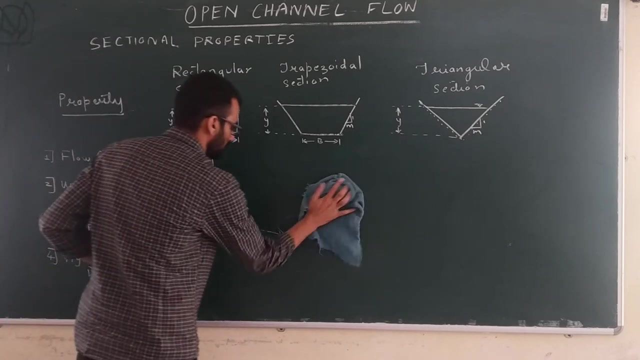 cross-section is there and flow is taking place. this is the depth. So, at the free surface, if you measure the width of the, If you measure this width of the free surface, Okay, At the top, then that will be the. that will be called as the top width. So for rectangular cross-section, hydraulic depth would be equal. 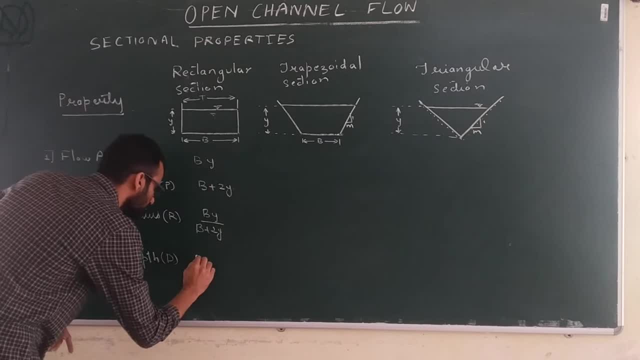 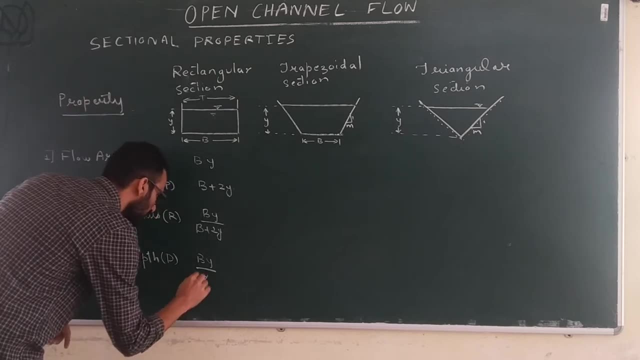 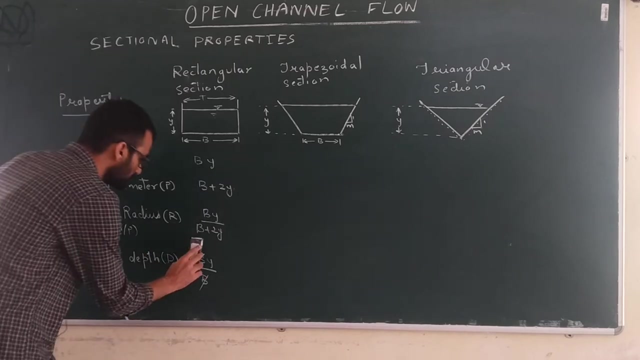 to A by T. So A is what B. Y upon top width is again equal to B. for rectangular cross-section it is B only, So B. B will get cancelled. and hydraulic depth is equal to the free surface, So B is the flow depth for rectangular cross-section. it will be how much It will be, just Y or flow. 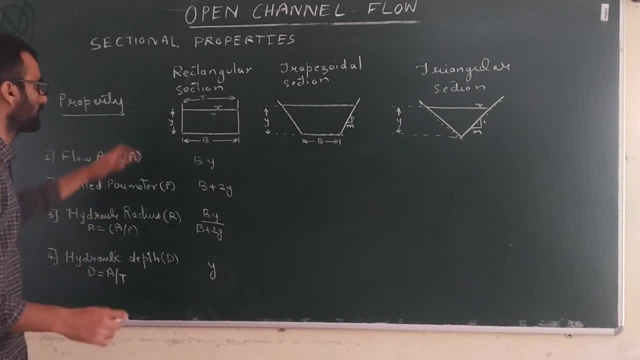 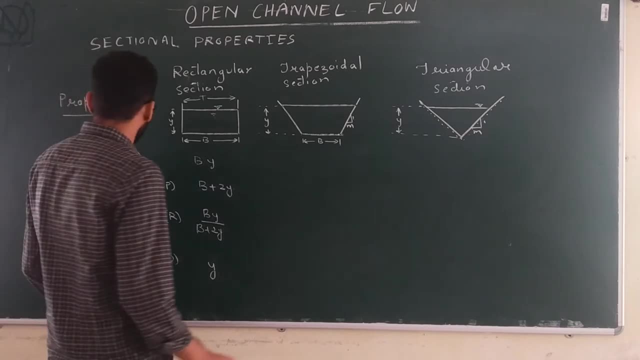 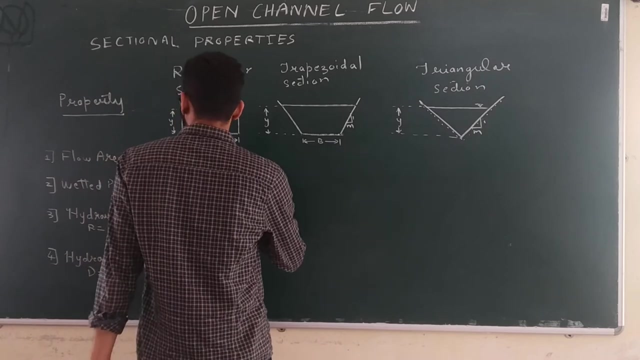 depth, because top width is equal to the base width here, and A by T. if you calculate you get only Y. Alright, Now the same flow sectional properties you can calculate for trapezoidal cross-section. Okay, So in trapezoidal cross-section, let us say, if you want to calculate the flow. 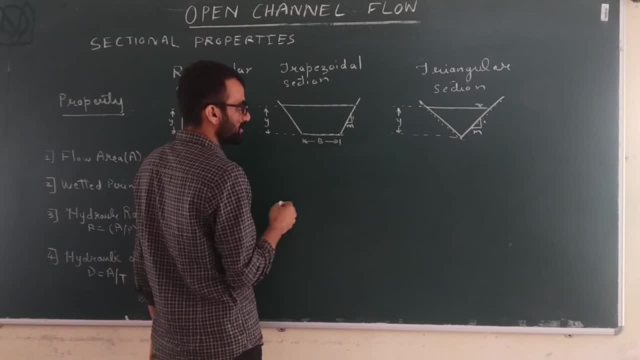 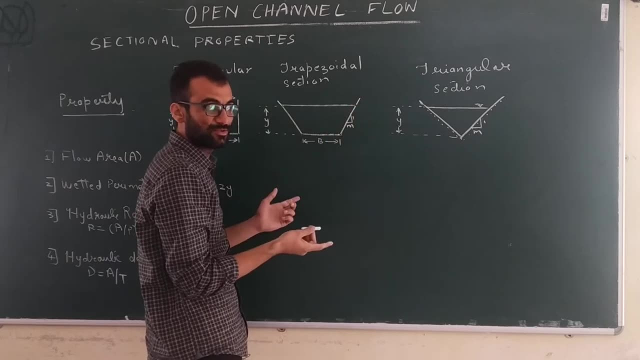 area. So what we will calculate? See to find the expression. the sides of the trapezoidal section are sloping. Okay, These are the two sides. They can have different side slopes. They can have same side slopes. Now I am considering the side slopes are same, How to denote the 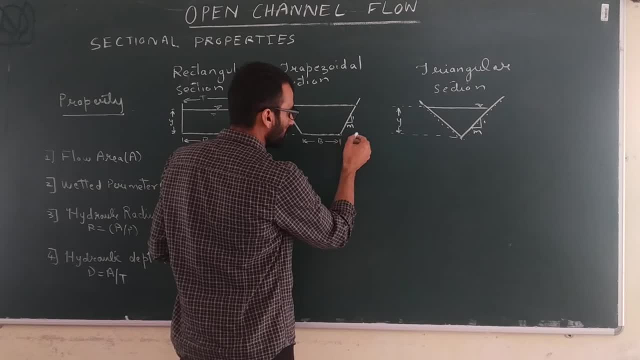 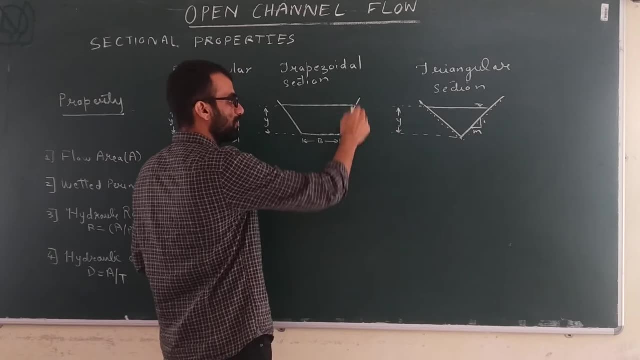 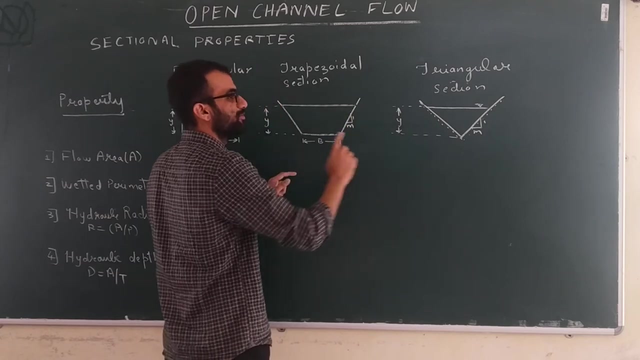 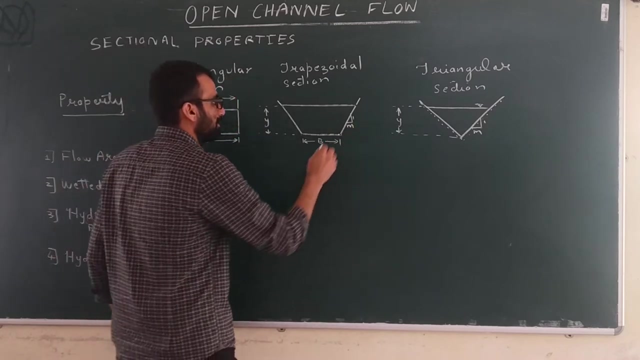 side slopes It is the horizontal distance which traced, which is traced to go up by one unit. Okay, So M horizontal, when you go For this slope, you get one unit of vertical distance. So this M is called as the side slope M. Okay, Now you see. if you want to calculate the flow area, then flow area is: 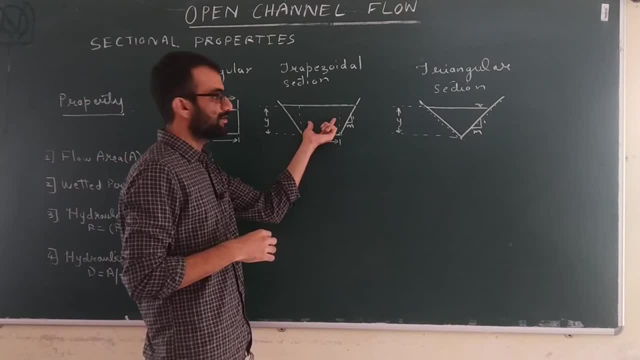 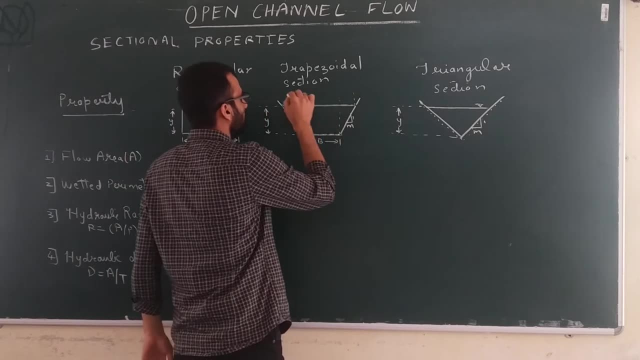 composed of this rectangular cross-sectional area also, plus this area of the two triangles. Okay, Now for area of triangles. you will need to calculate this length. Okay, How much will be this length? This length you can get from the trapezoidal cross-sectional area. 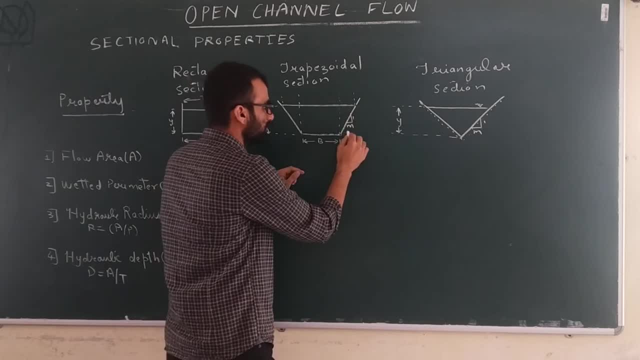 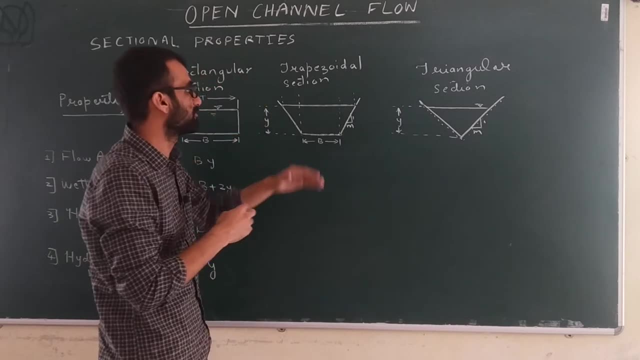 Okay, Now you see, if you want to calculate the flow area, then flow area is composed of this: sommes from the side slope. Okay, So in order to go one vertical, we need to travel M horizontal. So in order to travel by vertical, how much horizontal will have to travel? Just, 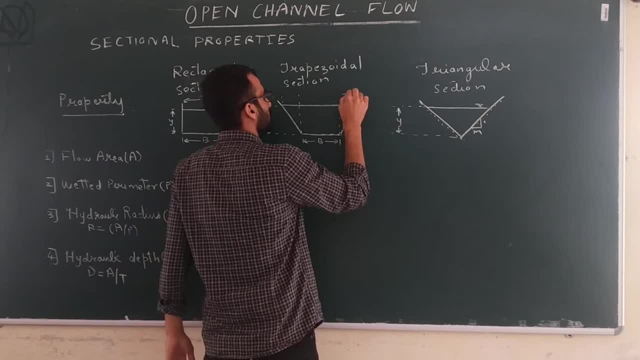 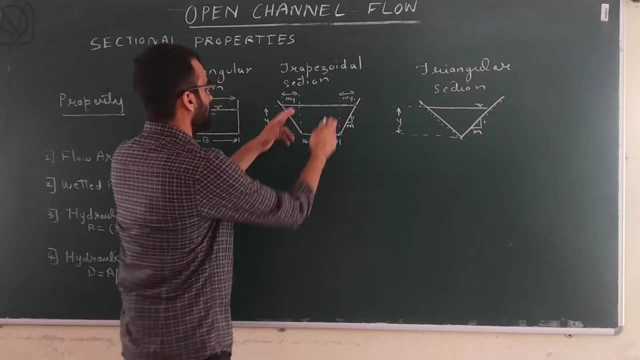 multiply it by M, So My, This will be My. Similarly, this also will be M into Y. This length, Okay, And this central part would be equal to v. Okay, So these are the lengths Now. flow area. flow area is area of this, these einige. So these are the lengths Now flow. area. flow area is area of this segment here. Okay, So you know the length which I put here, this same long insula. so this time I have to define equal to v. So if this length be the length of this segment here, then cut the length, V, okay, So this will be you know here. so 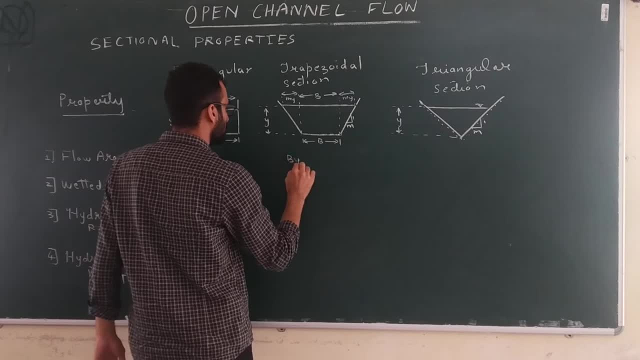 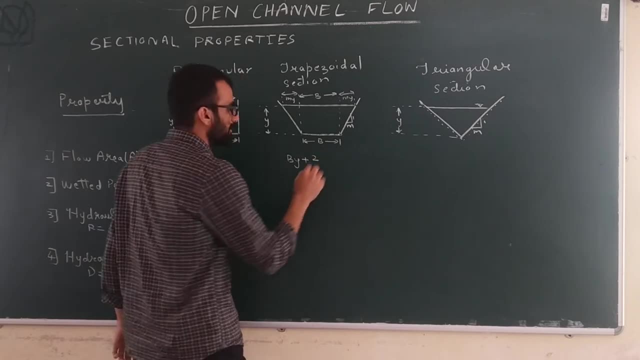 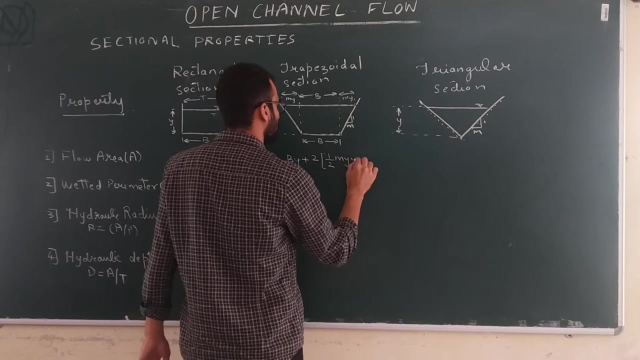 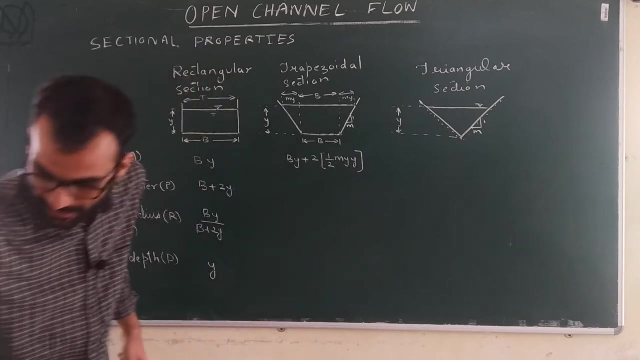 rectangle, that will be by plus area of this, two triangles, so two triangles and area of each triangle is half base into height. so half base is what my and height is y. okay, so this is your flow area. so 2, 2 will get cancelled and it will be my square. so directly you can write by plus. 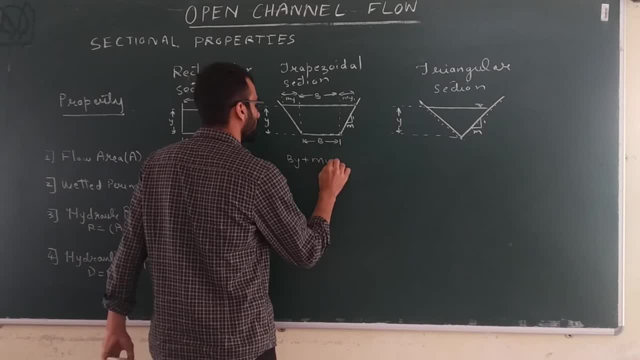 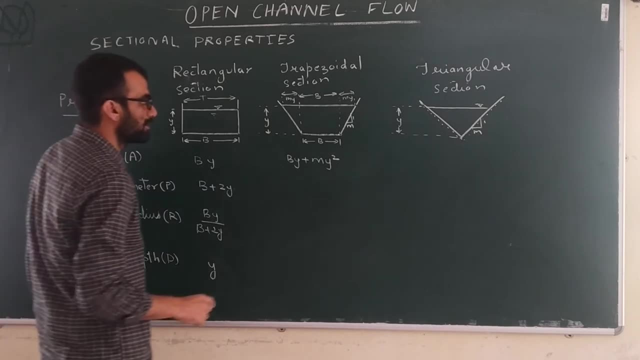 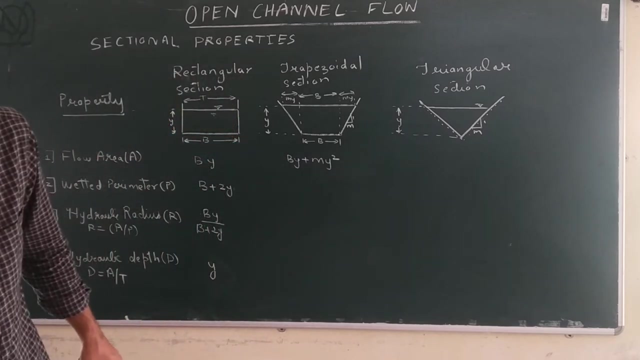 m y square. okay, this is your flow area of a trapezoidal cross section. now let's find out the wetted perimeter. okay, now, in this cross section, how much length is wetted by this flow? it is equal to, if you want to draw that length. 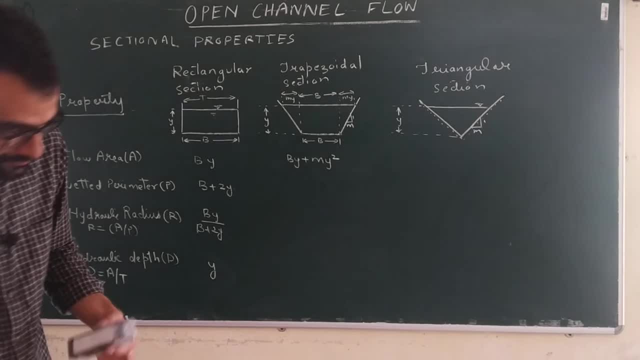 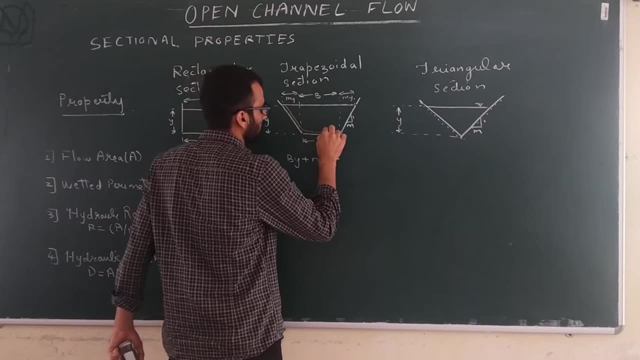 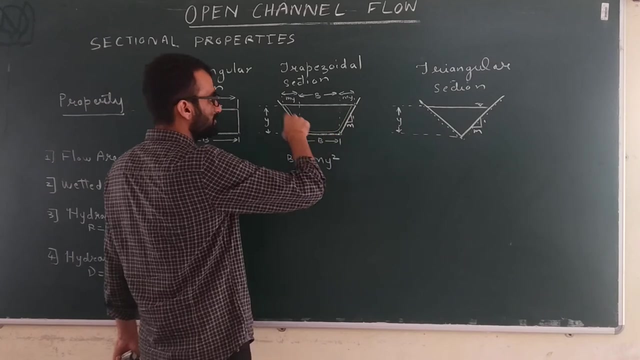 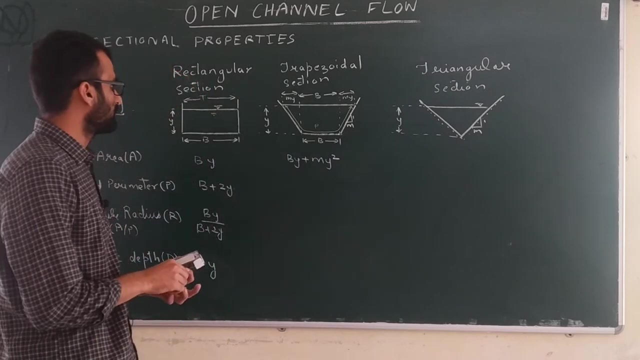 okay. so see, this length starts from here. it goes like this, and then it goes like this, and then, okay, good gain like this, okay, so this much length in the cross section is weighted by this flow. so this becomes your entire, becomes your weighted perimeter. okay, p, this becomes your p. now, how? 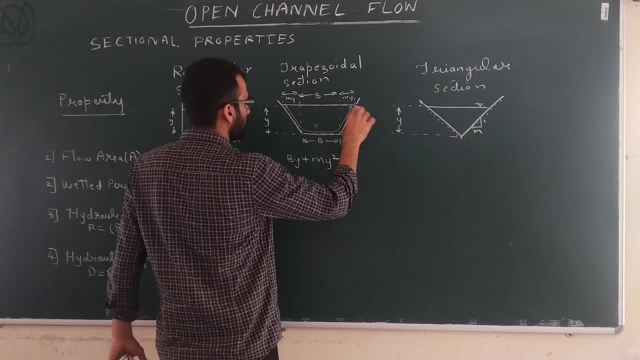 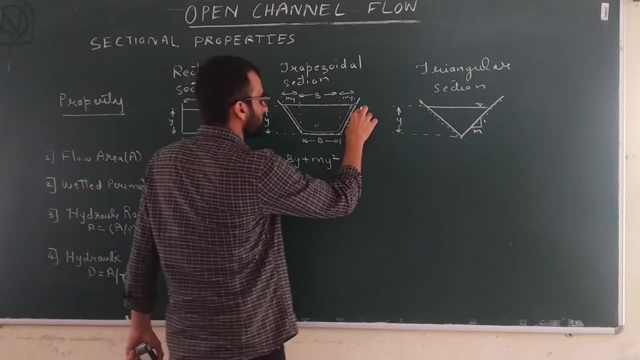 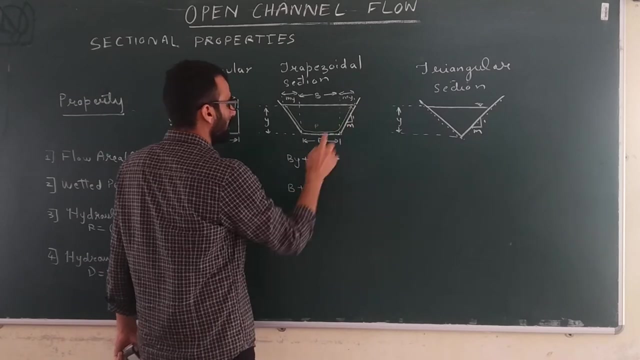 to calculate p. it is this length plus this sloping length plus this sloping length. okay, so this length is b base base weight is b plus now what is this sloping length? by trap, by pythagoras theorem, you can just calculate this hypotenuse plus and we have two hypotenuse. so 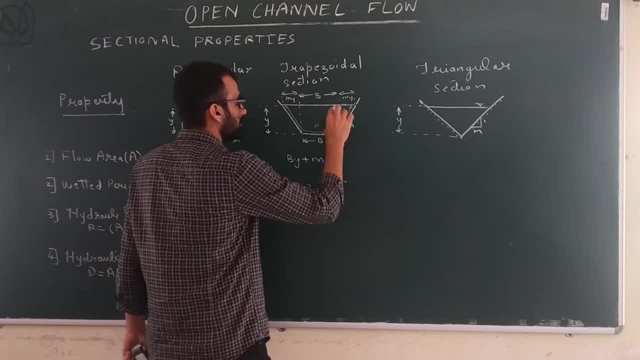 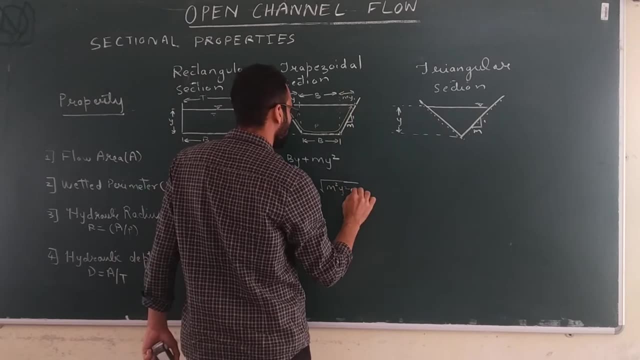 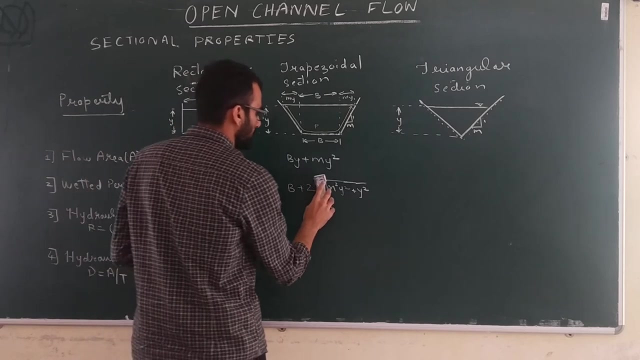 two times under root of this length of this square plus length of this square, so m square, y square plus y square. okay, so it will be equal to. you can just write: take y outside and you can write 2y under root, 1 plus m square. 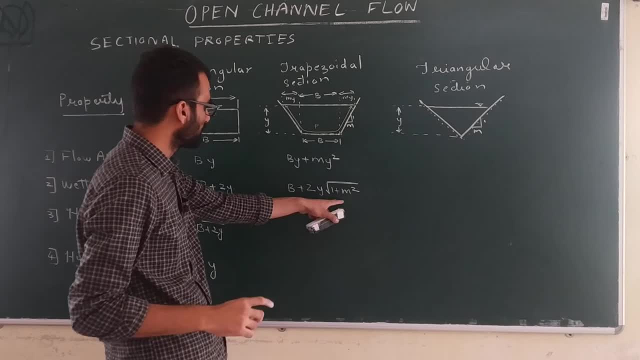 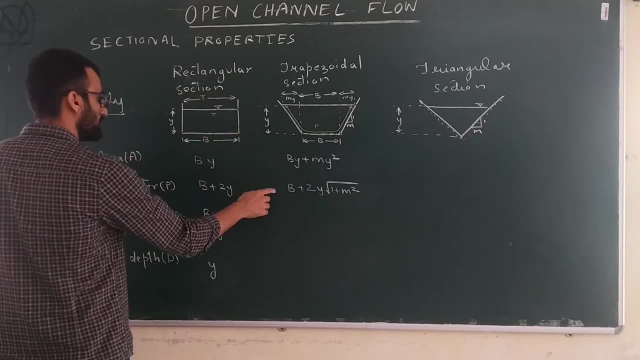 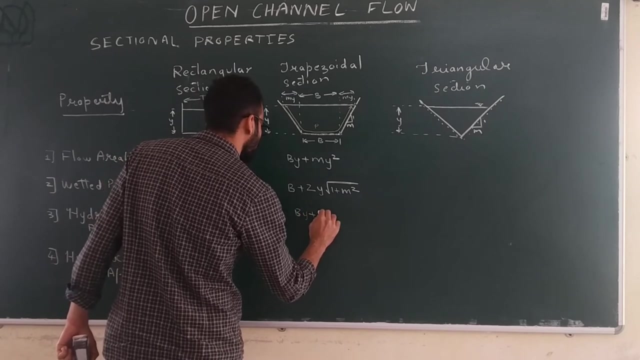 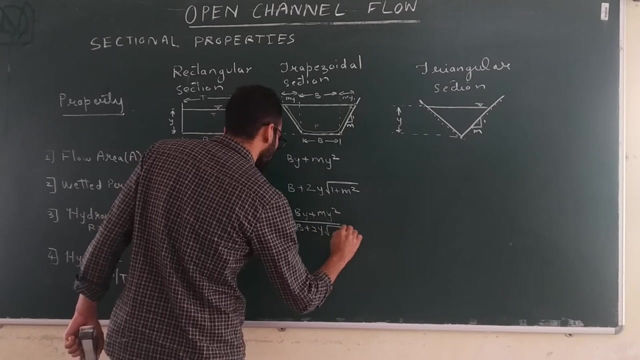 okay. so if you know the side slope, you know the base width, you know the flow depth, you can calculate this flow area and weighted perimeter. and once you know this flow area and weighted perimeter, you can directly get hydraulic radius. that is just divide a by p, so by plus m y square upon b, plus twice y under root, 1 plus m square. okay. 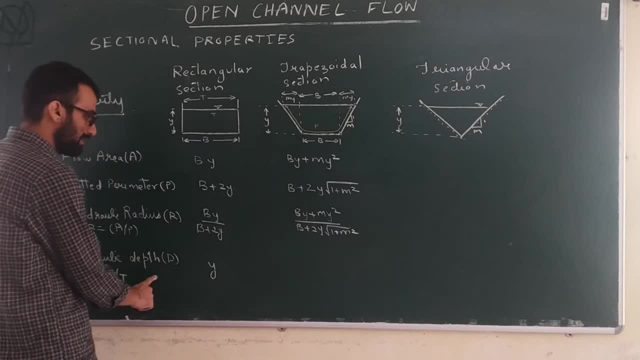 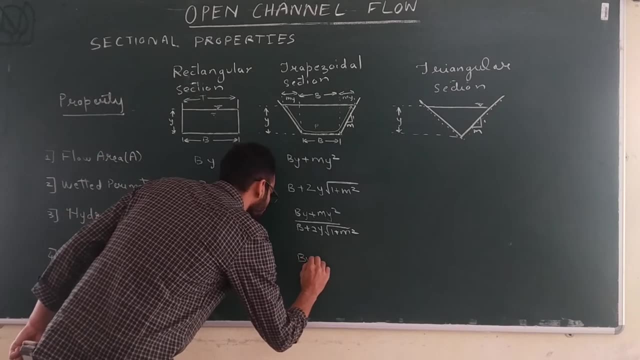 now, what will be the flow depth of this perimeter? okay, so if you know the side slope, you know the hydraulic depth. again, hydraulic depth is the ratio of flow area divided by the top width, flow area and top width. so flow area is again by plus m, y square upon. 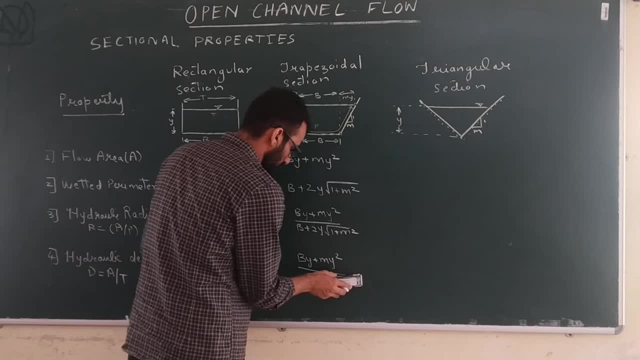 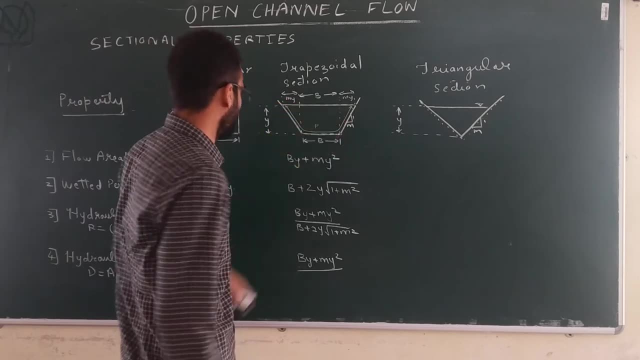 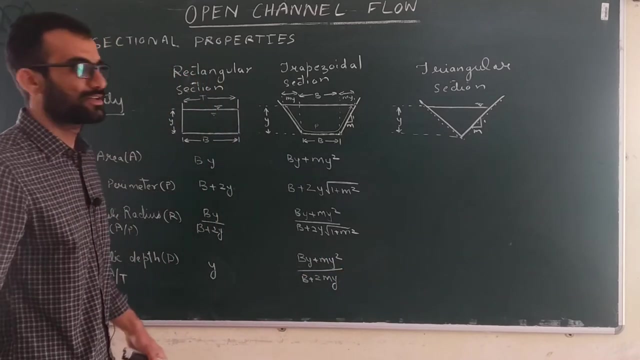 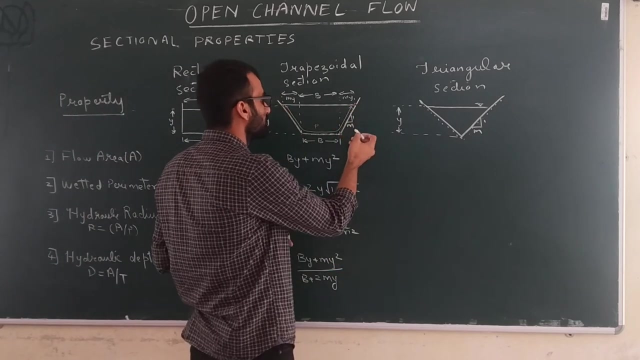 now what is the top width? so top width is b plus this length, plus this length, so b plus twice m y. so this is your hydraulic depth, mean depth or hydraulic depth. simply Now see if you have different side slopes. if you get a problem in which you get different side slopes, you can calculate each area of each triangle. 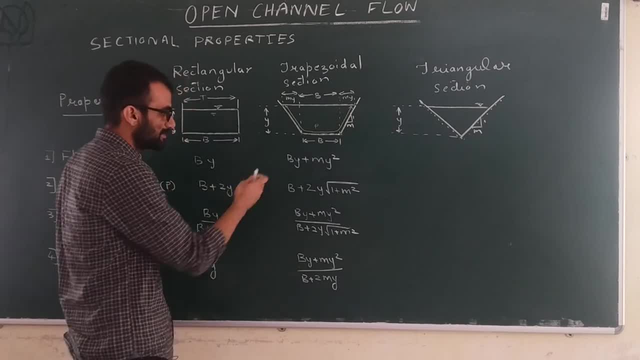 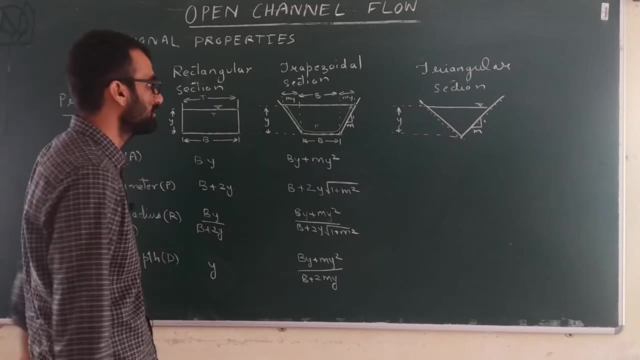 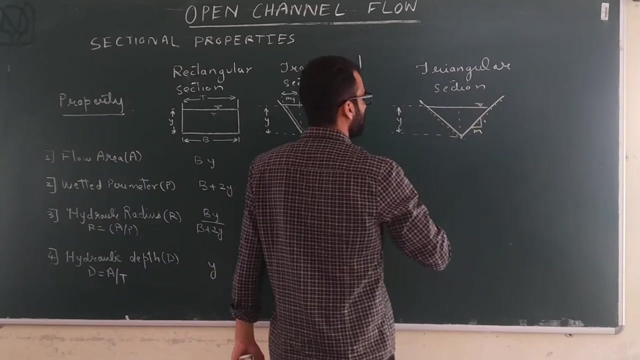 separately. and then you can go for calculation of flow area and similarly for the wetted perimeters also. So in this way you can find out the properties of a trapezoidal section. Now let us see for a triangular section. So for triangular section, there we have two triangles. 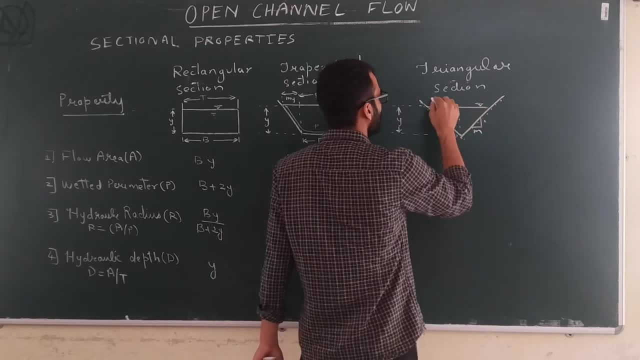 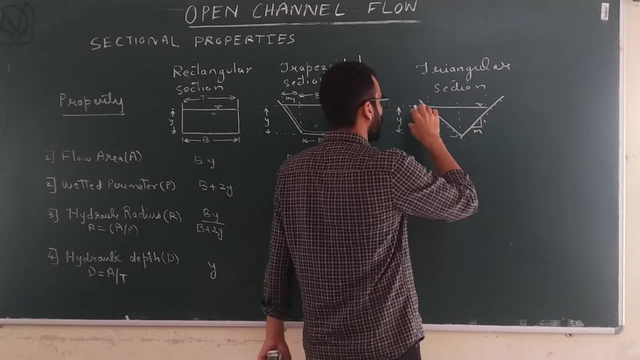 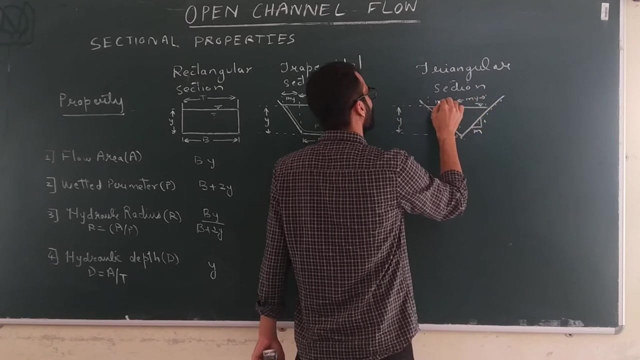 okay, this left and right hand side triangle we have. okay. So what are the lengths here at the top? what will be the length For one vertical? we have to travel m horizontal. So for y vertical we will have to travel how much horizontal m into y. okay, This is my. I mean, this will be also my. 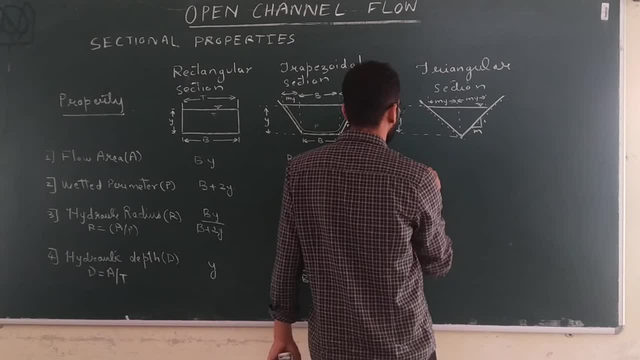 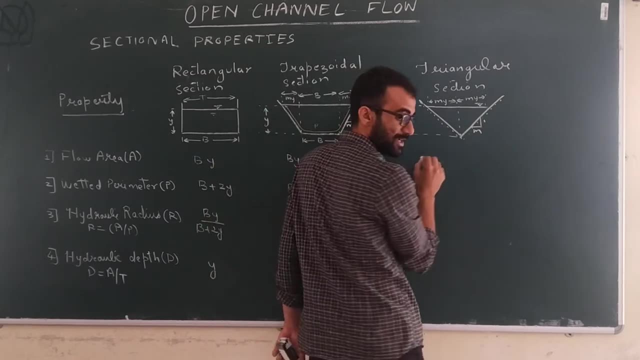 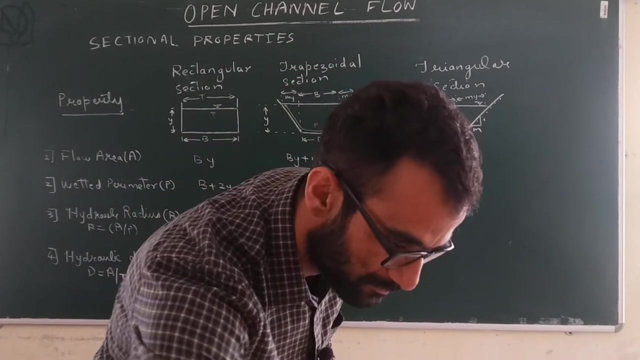 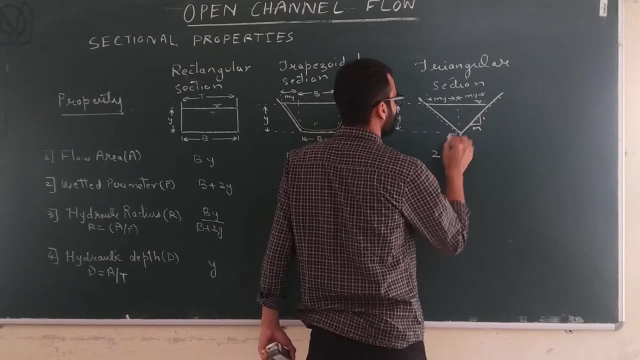 okay, Now what will be the flow area? It will be the addition of these two triangles, area of these two triangles. So just add the area of these two triangles. so twice okay, So two times the area of this two, this triangle. so half, two times half. base is what m, y and height. 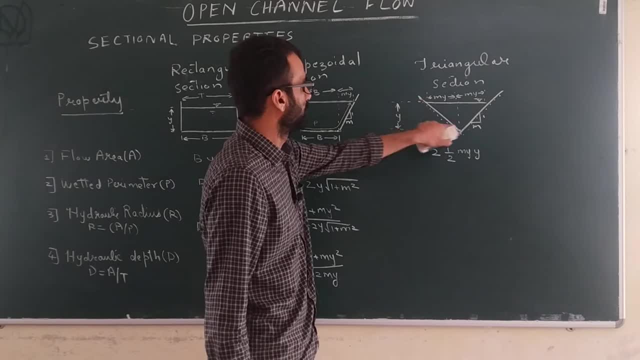 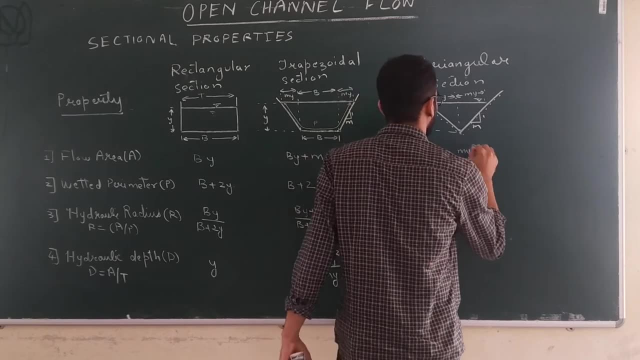 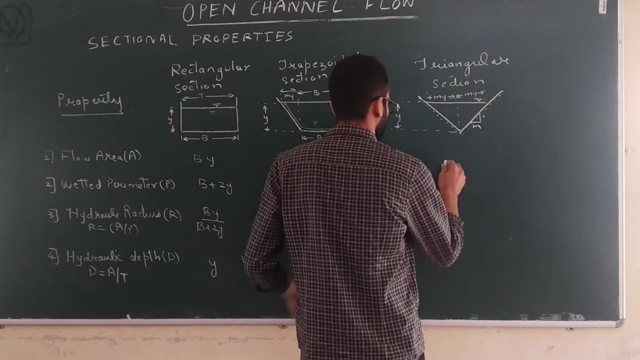 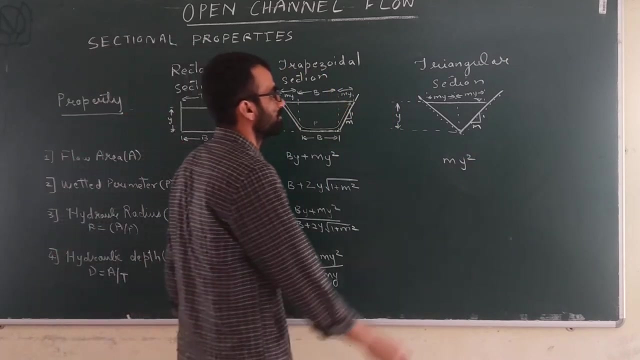 is what y? So this is the flow area. So 2. 2 will get cancelled, we will get m y square. Okay, this is the flow area of a triangular section. Okay, what will be the wetted perimeter? So just add that these two hypotenuse these two sloping lengths, So two times the sloping lengths.